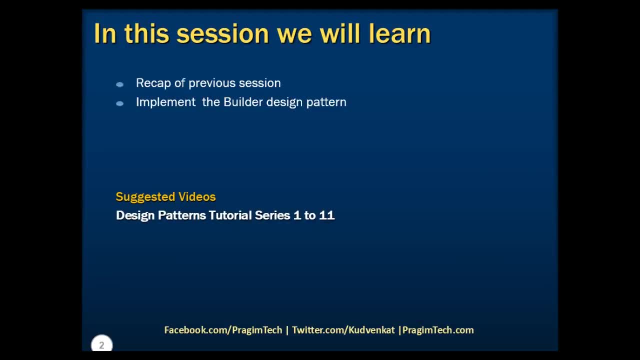 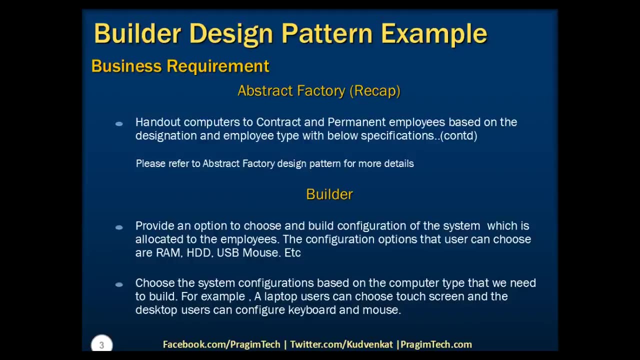 the tutorial before proceeding. In the previous session we have implemented the business requirement of configuring the systems allocated to the employees without using any design patterns. Now let's assume that we have a new requirement of choosing the system configurations based on the computer type that we need to build. Let's say we need to. 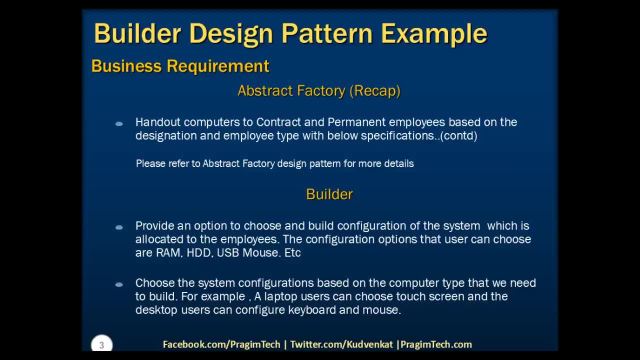 choose different type of configurations for the laptops and desktops that are allocated to the employees. For example, a laptop user can choose touch screen as a configuration for a graphic layout which is limited to two configuration, whereas desktop users can configure keyboard and mouse, As discussed earlier. 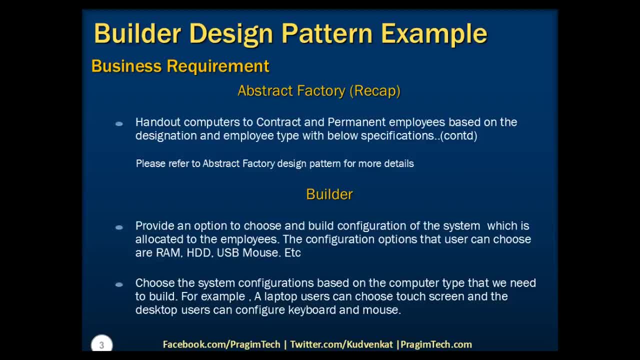 the current implementation, which we adopted in the previous session, becomes complex and complicated if we do not choose any creational design pattern over here. In our case, since we are building the system configuration in a step-by-step process, build a design pattern suits our requirement. First, let's see how we can migrate the current 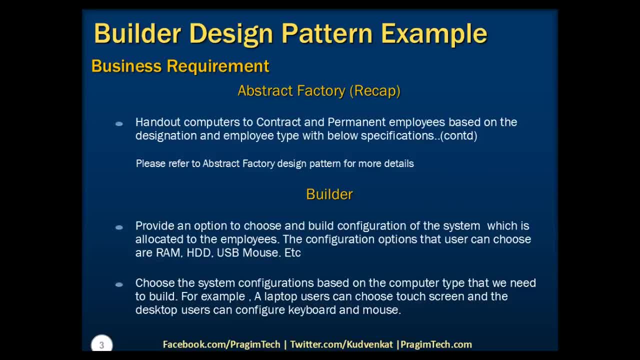 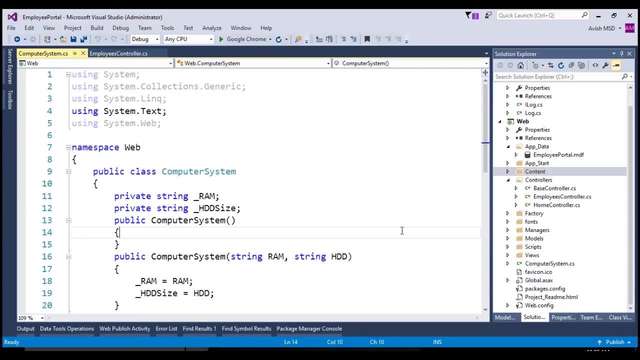 code to the Builder implementation. Once it is achieved, we will address the additional requirements as mentioned here. Let's now switch to Visual studio and implement the solution using our previous working example. Let's start decoupling the ComputerSystem class that we have built in the previous session of Builder design pattern. 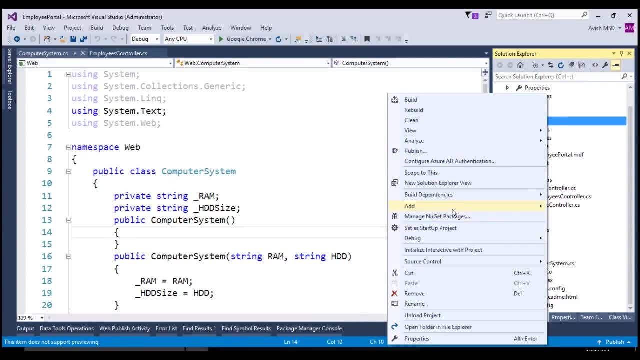 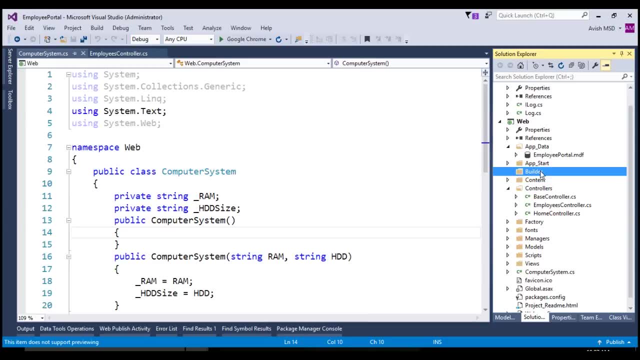 First, let's create a folder Under this web project, add new folder and name this folder as builder. let's create another folder under this builder folder, add new folder and name this folder as product. the end product that we are going to build is the computer system, and we have 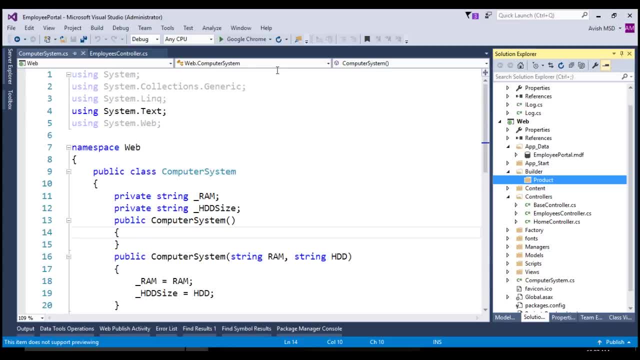 already created computer system class in the previous session. let's move this computer system class to this product folder. let's create another folder under the builder folder, add new folder and name this as I builder, which holds the interfaces related to the builder design pattern. let's create, add new item and. 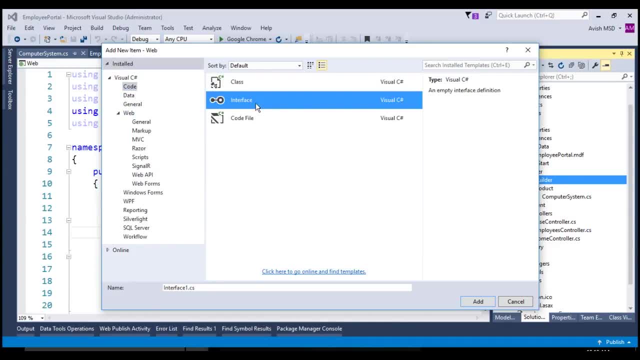 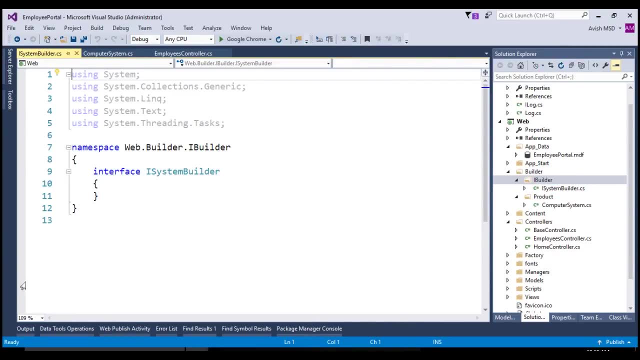 let's add an interface and let's name this interface as I system builder, since we are building the system configuration, we are choosing the system configuration and we are choosing the system configuration using the name as I system builder. on other note, to simplify the builder design pattern explanation and to match the explanation with the representation. 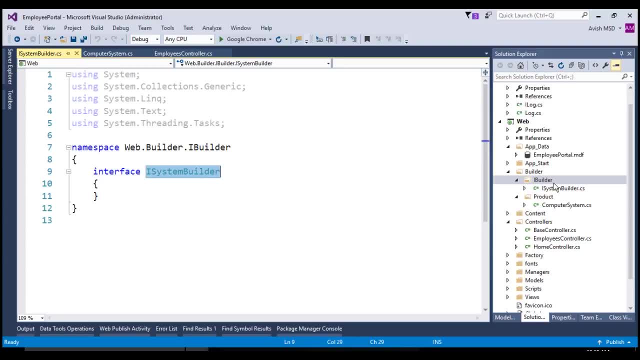 diagram that we have used in the previous session and following this folder structure. however, please feel free to come up with your own way of defining the classes based on your requirement. the main purpose of this I system builder is to build the system in a step-by-step process and finally, 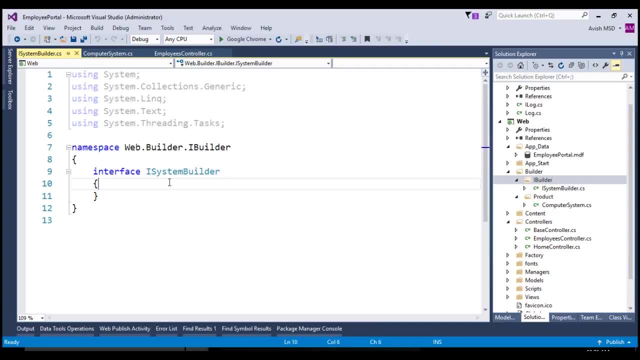 it should return the object once it is built, let's say, while building the system, we need to add memory. so let's create a method, interface method- void add memory. let's pass the parameter as memory. let's create another method to add drive size- void add drive- which accepts the drive size as the input parameter. 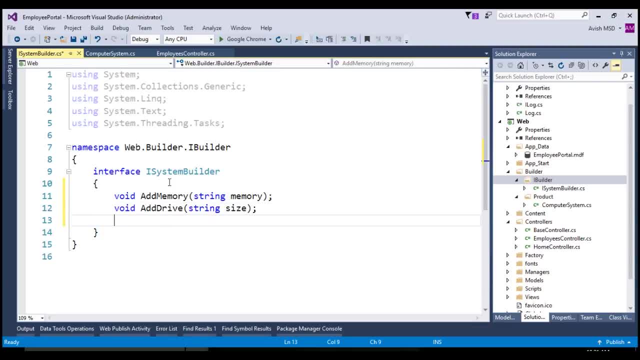 once the builder builds both of the required configurations, and then we need to return the build system, which is our computer system. so let's add another method which returns computer system and name this method as get system. let's now switch to the computer system and eliminate the constructor with parameters. 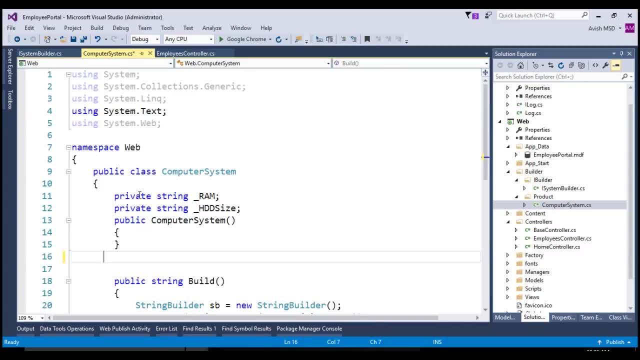 and change these private properties to public so that these are set from the concrete builder classes. let's change this to public. let's also remove this underscore RAM and rename this as RAM, and let's set the properties for this RAM as get and set so that it becomes a public variable. let's also change this to public. 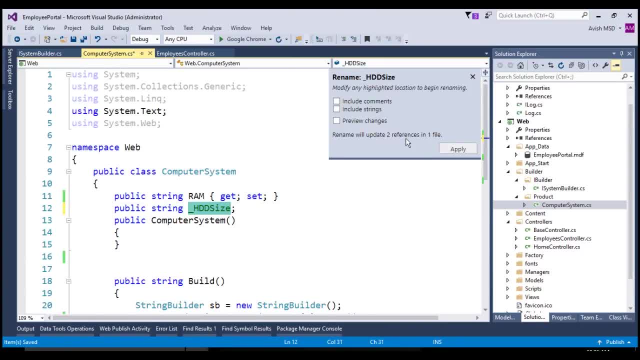 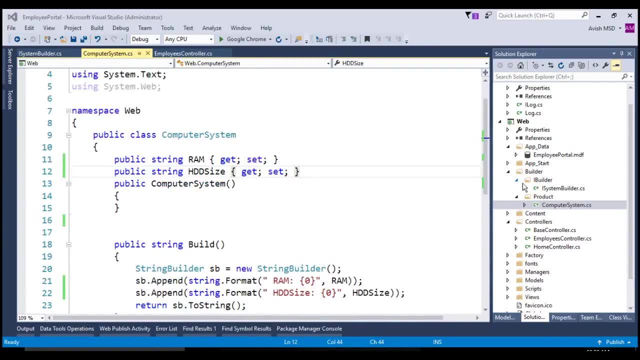 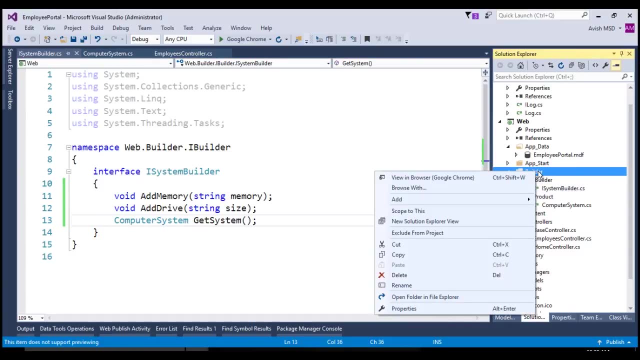 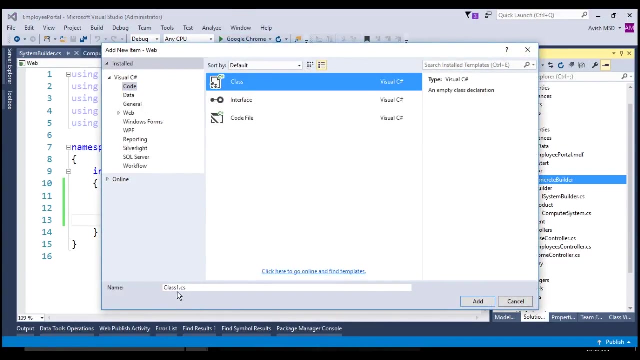 and rename the property, the size, remove the underscore and assign, get and set properties for this. let's now add concrete builder classes, which implements the isystem builder. right click on this builder folder, add new folder and name this folder as concrete builder. let's add a class: add new item, choose a class and name. 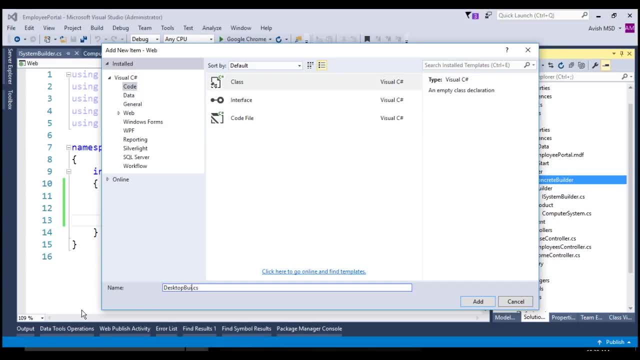 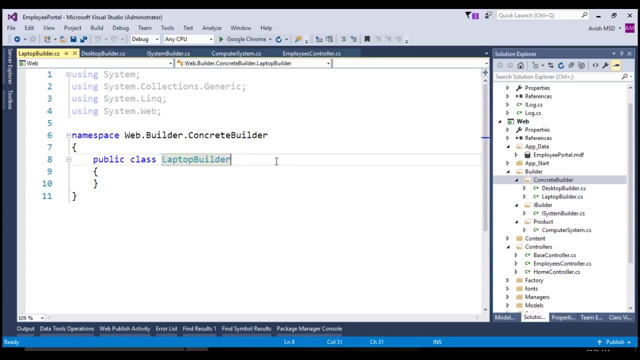 this class as desktop builder. let's add another class. add new item. choose the class. let's name this class as laptop builder. let's inherit the interface: isystem builder. let's resolve this issue by using webbuilderibuilder. let's also implement the interface methods. implement interface. 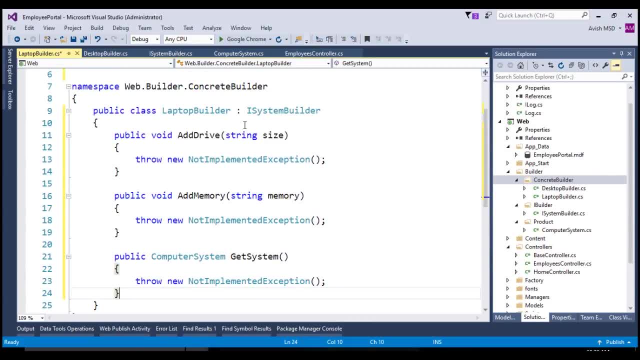 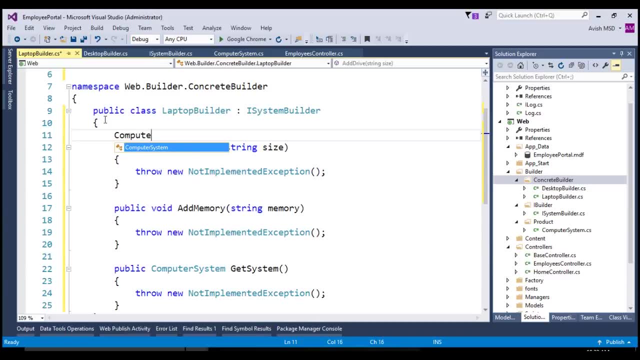 the purpose of this laptop builder is to build the system configurations and return the computer system which is being built. so let's create a computer system object, computer system object and name it as laptop, since we are building a laptop equal to new computer system. in the add drive let's say laptop dot. HDD size equal to size. 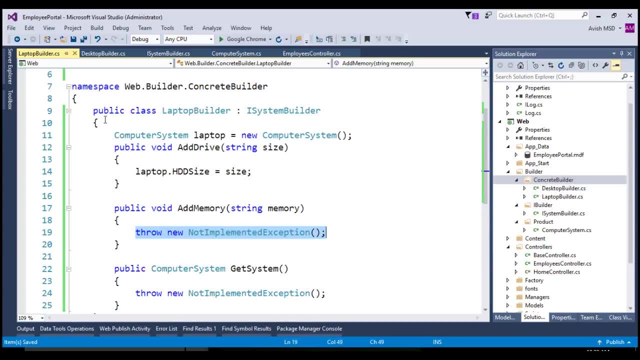 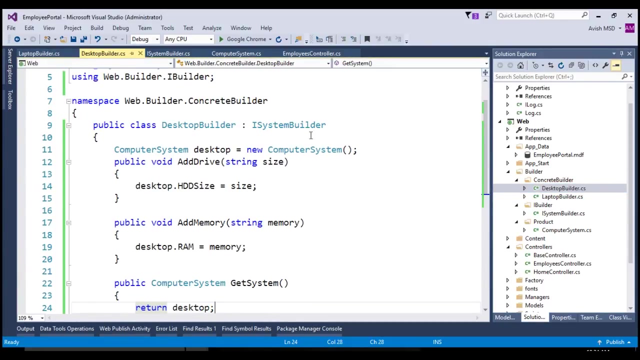 let's assign the properties for the laptop. for memory, it will be laptop dot RAM equal to memory. once these two configurations are built, let's return the laptop here. return laptop. let's now switch to the desktop builder and implement the isystem builder. to make the things faster, I have already implemented the isystem builder in the desktop builder class. 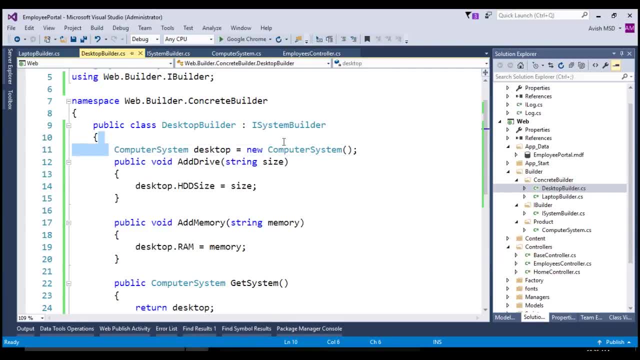 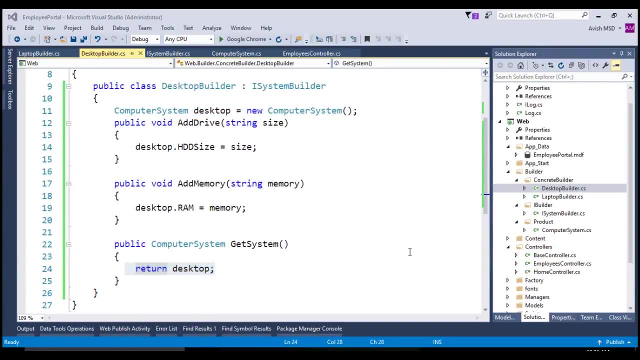 the only difference is we are building a computer system which is a desktop over here, and we are returning the desktop once the configurations are built. now, as per the enhanced requirement, let's say to provide an option to add keyboard and add mouse as the configurations for desktop. 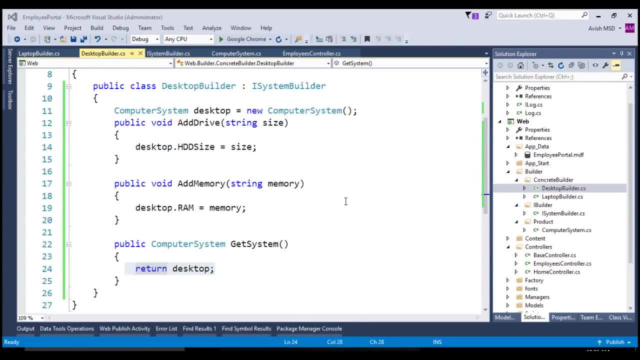 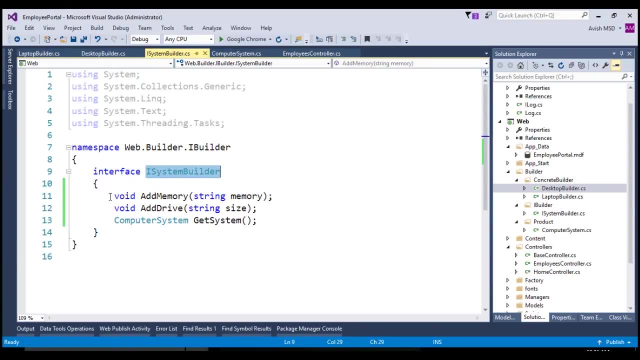 and we need to add touch screen as a configuration for laptop. let's switch to the isystem builder. notice that adding memory and drive are the common configurations for both desktop and laptop. let's add few more methods to the isystem builder to address the enhanced requirements. 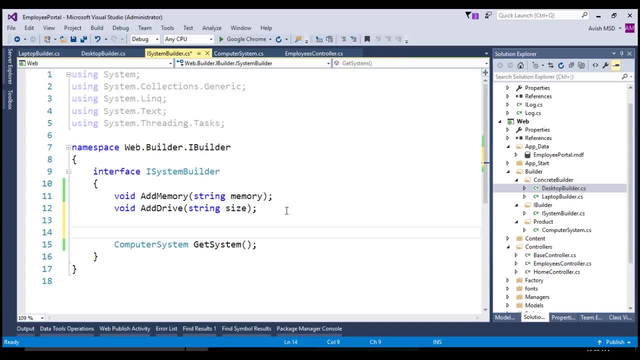 for desktop. let's say we need to choose the type of keyboard and mouse, which should be either wireless or a regular usb mouse. so let's add those methods as void- add keyboard and which accept string type as the input parameter. let's also say add void- add mouse. 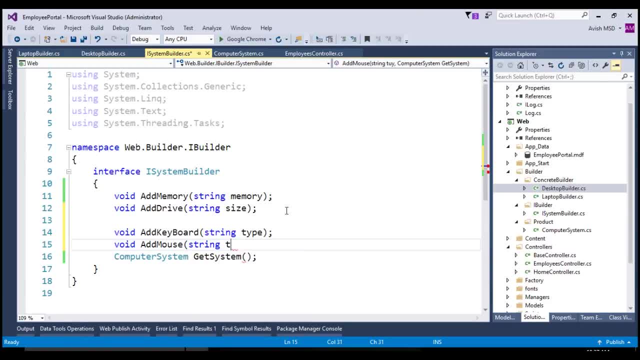 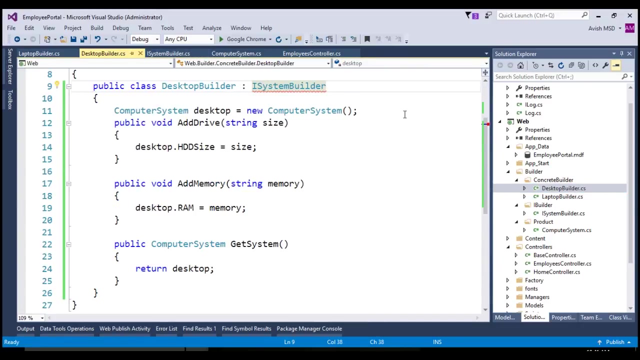 which accepts the type of the mouse as input parameter. let's now add another method: void- add touch screen with input parameter as string enabled. it says whether the touchscreen is enabled for the laptop or not. let's now switch to the desktop builder and notice that isystem builder is showing a. 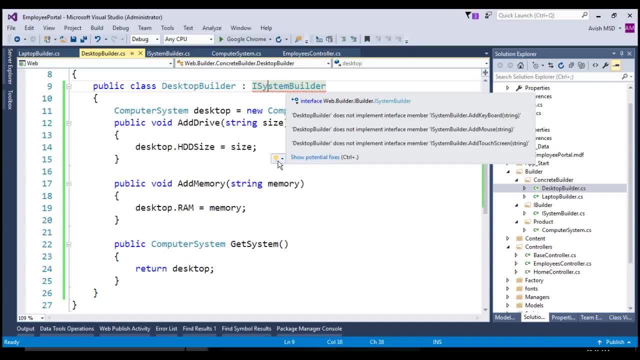 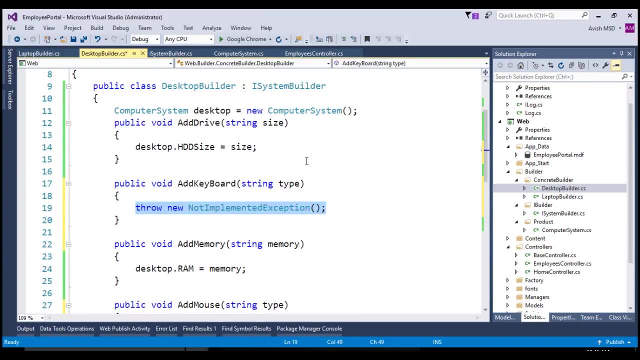 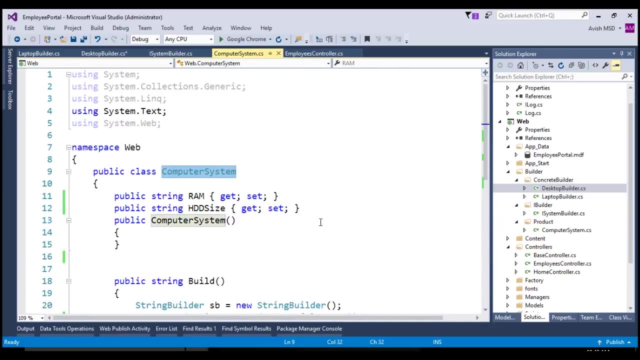 compilation error. so let's fix this error by implementing the missing methods. now, in the add keyboard, we need to assign the keyboard type. to assign the keyboard type for the computer system, let's switch to the computer system and add properties to the computer system. the properties would be string keyboard. 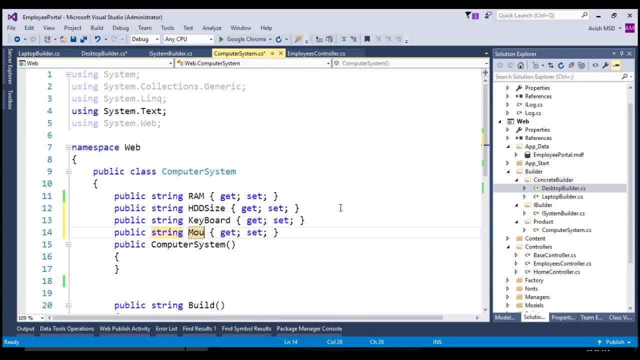 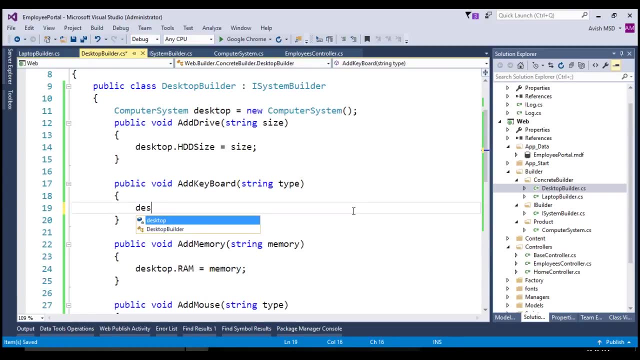 add another property string- mouse. and let's add another property string: touch screen. let's now switch back to the desktop builder and assign these properties here. let's say desktop dot keyboard, equal to type of the keyboard. let's also do the same thing for add mouse as well. 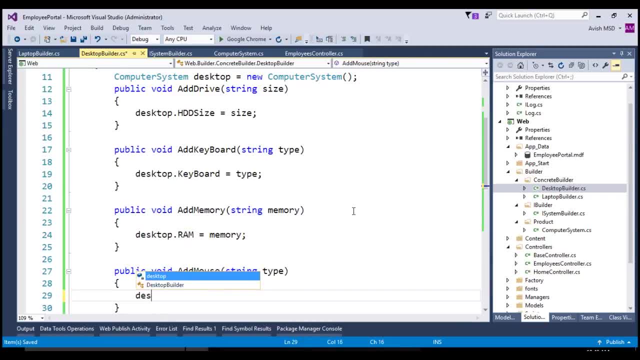 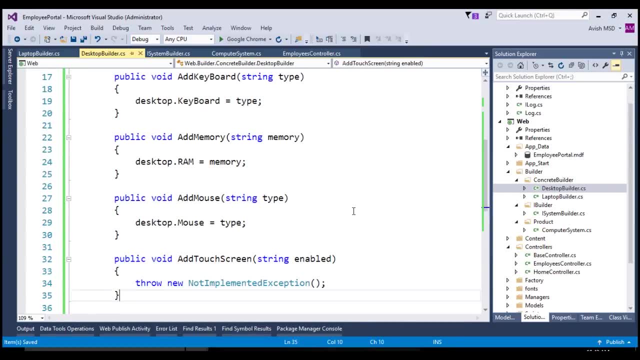 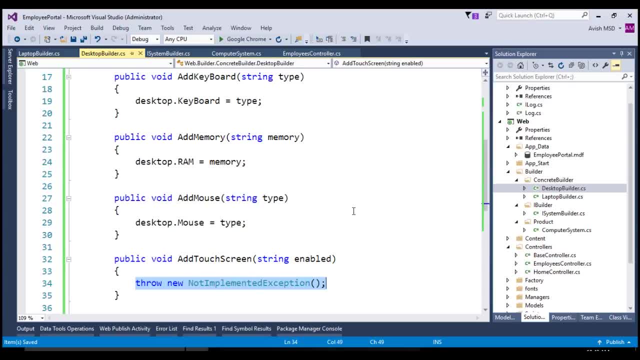 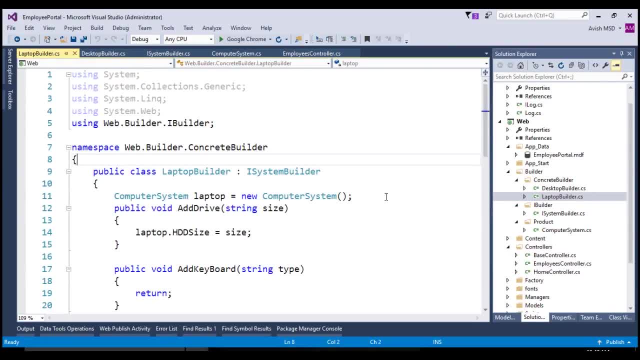 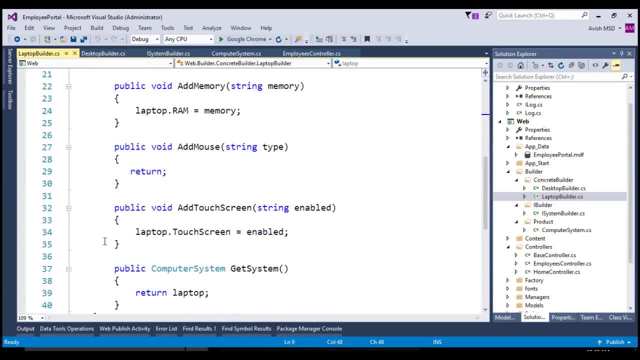 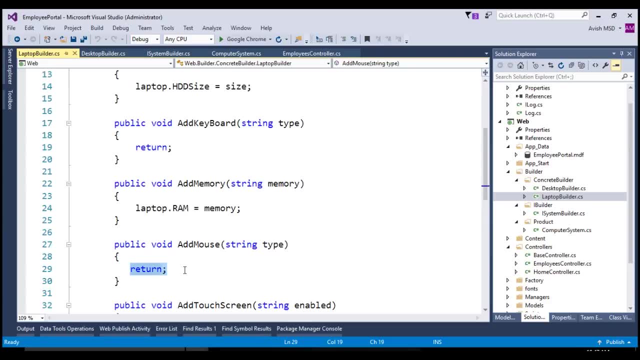 Notice that I have added touch screen as a property and using a written statement for keyboard and mouse. as it doesn't make any sense using keyboard and mouse for a laptop builder, Let's create another class that controls the way builder is executed. In some situations, building a product has to follow specific steps and the class that 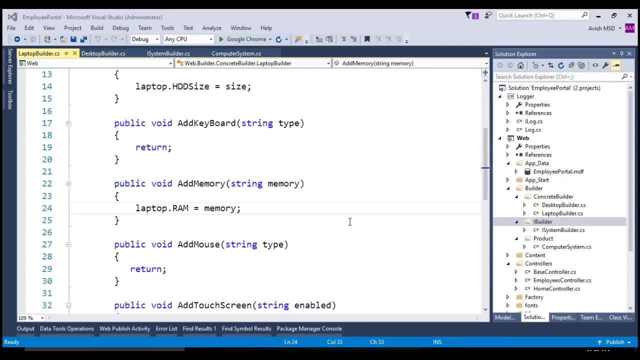 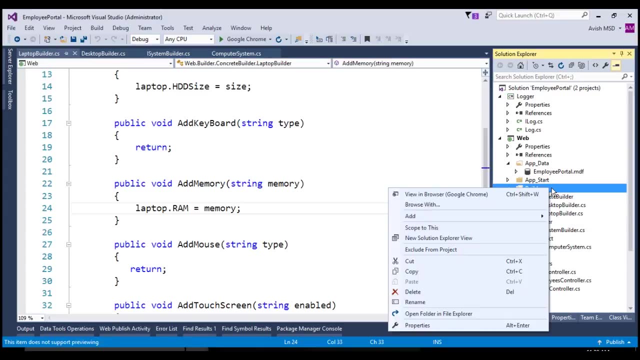 directs those specific way of execution is called director. Let's create a folder called director that builds the system using ISystemBuilder and the collection of parameters that's being passed. Let's create a folder in a class: right click, add new folder and call this folder as director. 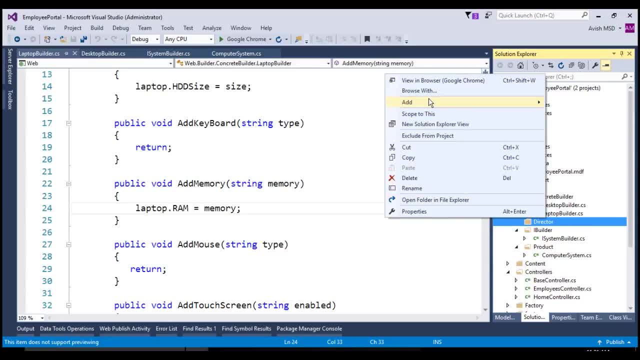 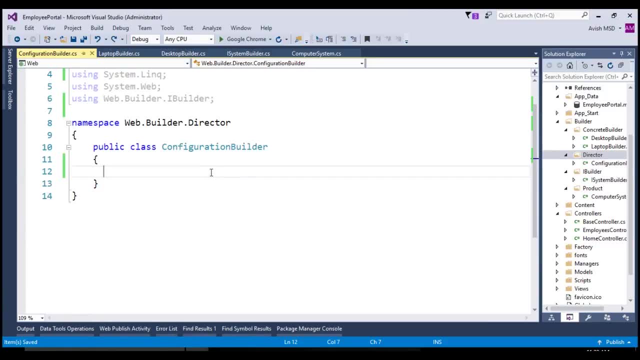 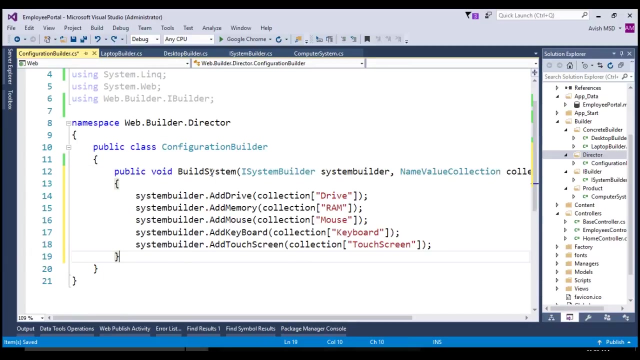 and let's add a class. right click, add You are- And call this director class as configuration builder. Let's add a method build system with ISystemBuilder and name value collections as the input parameters. To make the things faster, let me copy the code which have already written from my notepad: 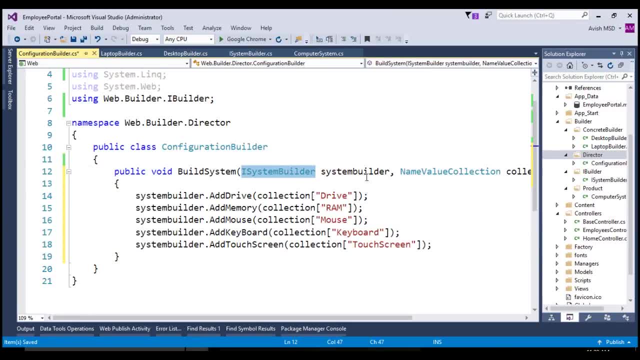 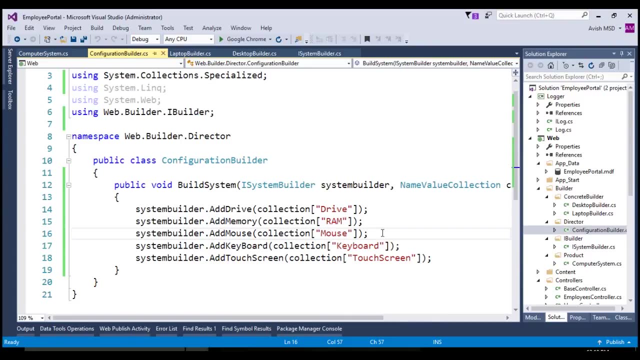 The ISystemBuilder is an interface which represents either the laptop builder or desktop builder in the runtime, Whereas the name value collections are the configuration chosen for these concrete builder classes from the front end. Now that we are building the system in the configuration builder, let's switch to the 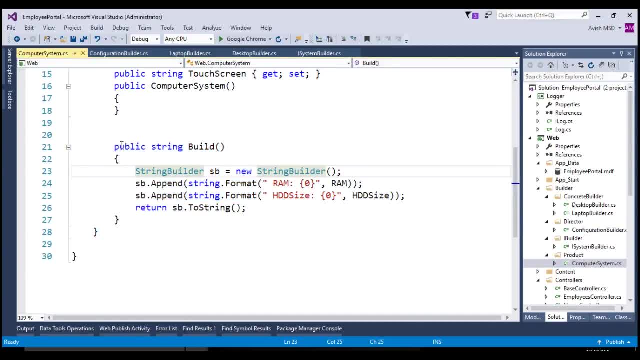 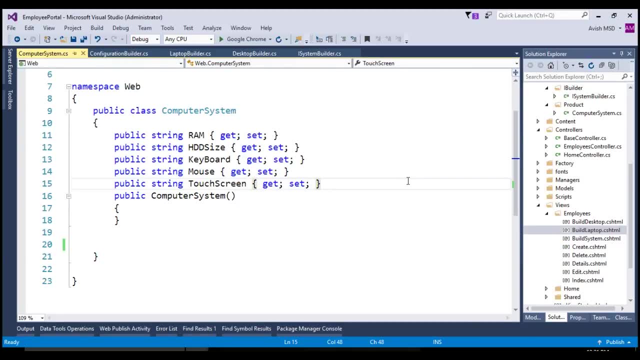 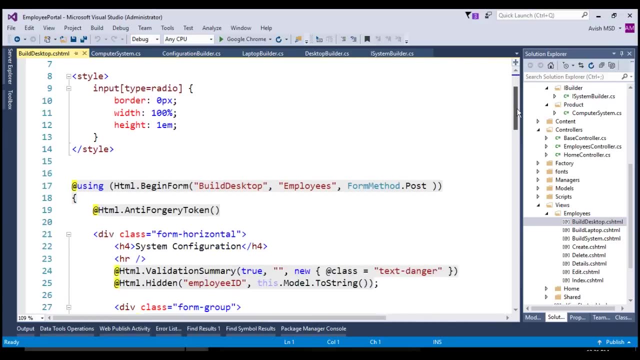 computer system and remove the build method that we have created in our previous session. To make the things faster, I have created two views for laptop and desktop under the employees view folder. Okay, Okay, So for the two view types I have provided an option to choose the touch screen in the 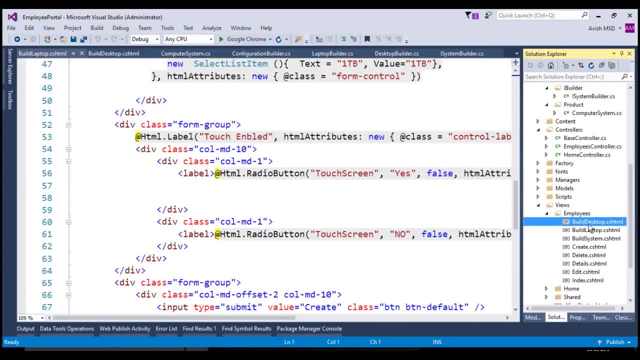 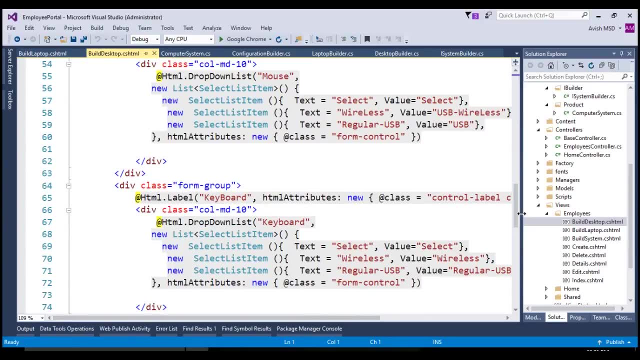 laptop view, Whereas in the desktop view I have provided an option to choose keyboard and mouse types. You may be wondering why we need to create two new views. to answer that, it's not mandatory to create two new views and we can leverage on creating these two system types as partial. 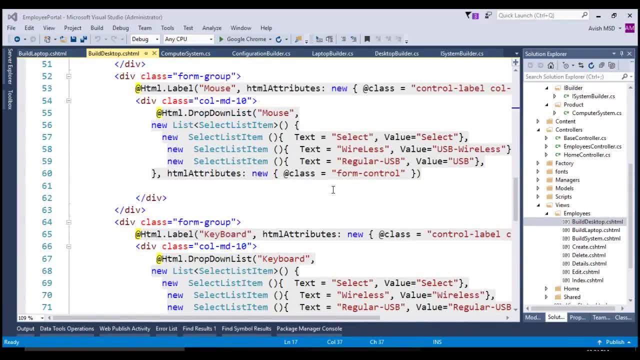 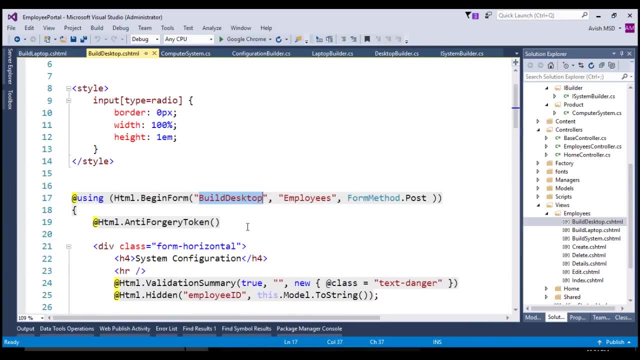 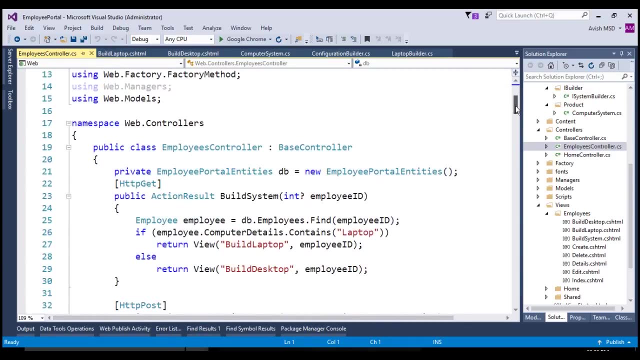 views and embed them in the main building. However, to make the things simple, I have created two new views Now on submit click. we are submitting the views to the respective controllers. Let's switch to the employees controller To make the things faster. notice that I have already enhanced the build system action method. 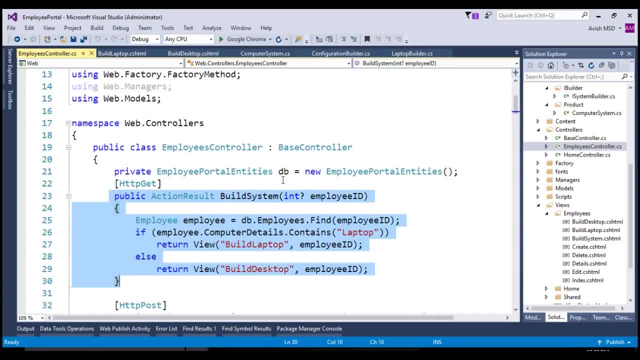 which we have created in the previous session. The build system will return the respective views of desktop and laptop based on the build system action method. The build system will return the respective views of desktop and laptop based on the build system action method, Based on the system type allocated to the employees. 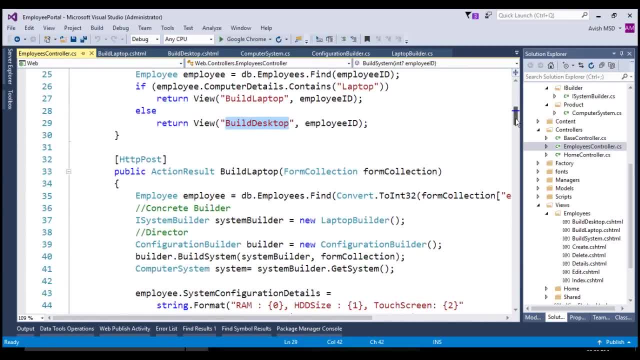 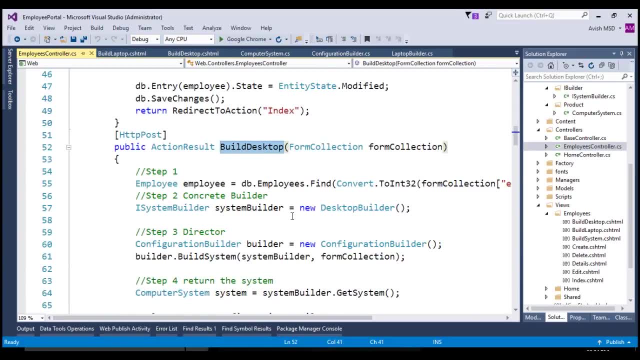 I have also added two new action methods, which are build-laptop and build-desktop. Let's take a closer look and inspect the code of the build-desktop action method that have already created. Notice that in the first step, we are retrieving the employee details, and in the second step 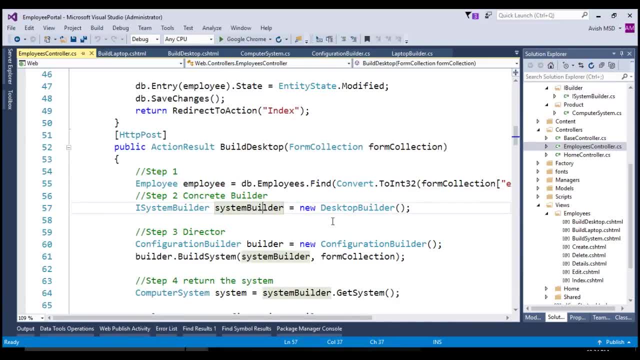 we are creating the instance of the system builder, which would be either desktop builder or laptop builder. we are creating a desktop builder here. in the third step, we are creating the director object and passing the concrete builder and the form collection, which is a configuration chosen from. 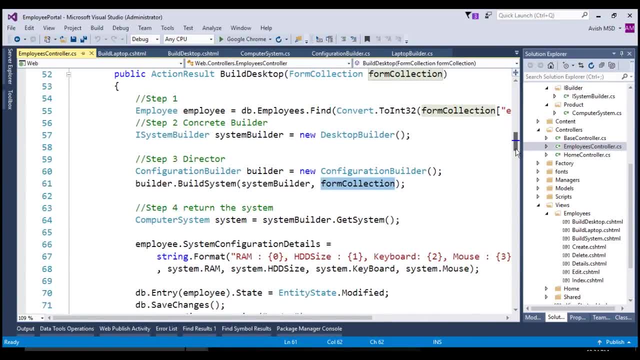 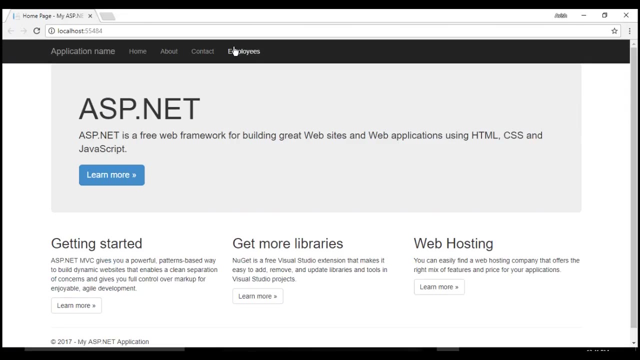 the respective view. the director is responsible to build the system, and once that is done, in the fourth step we are returning the computer system which has the details assigned as the properties. at the end, we are saving the configurations to the system. configuration details- column of the employee table. let's now run this application and see these changes in action. let's choose: 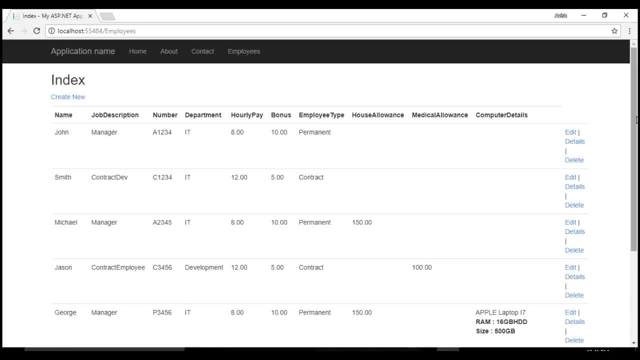 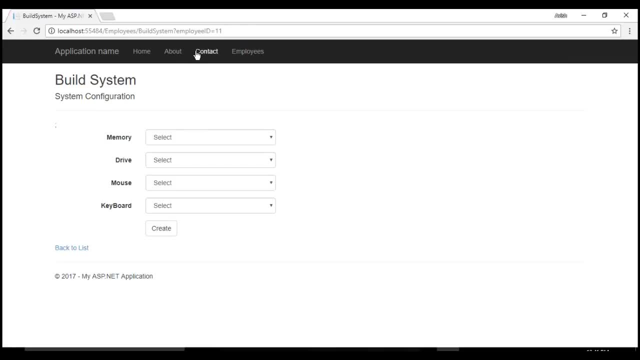 employees tab. let's click on build system of sebastian who has got desktop. notice that the moment we click on the build system, it is presented with a desktop view. let's the memory: 16 gb drive as 500 gb, mouse as a wireless mouse and keyboard as a regular usb. 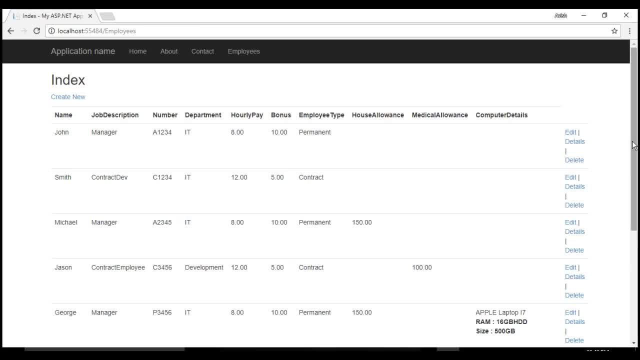 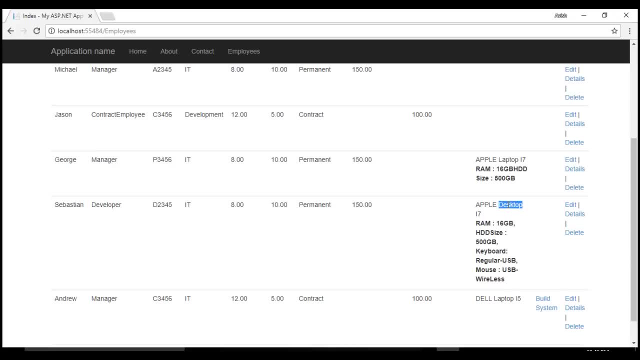 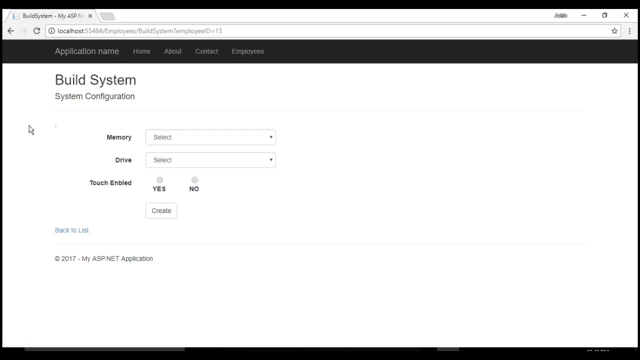 keyboard. let's click on create. look at that. we have successfully built the configuration of the apple desktop, which is allocated to sebastian. let's do the same thing with andrew, who is the manager. let's click on the build system. look at that. we are presented with the laptop view. let's